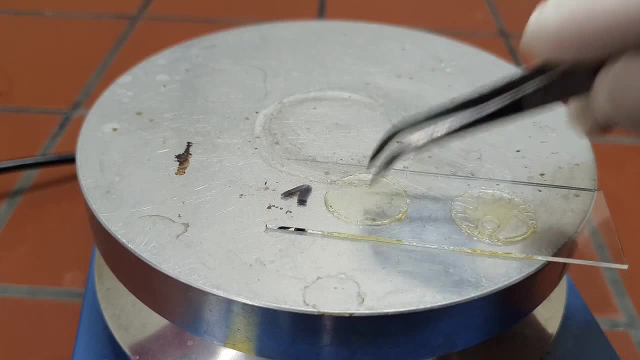 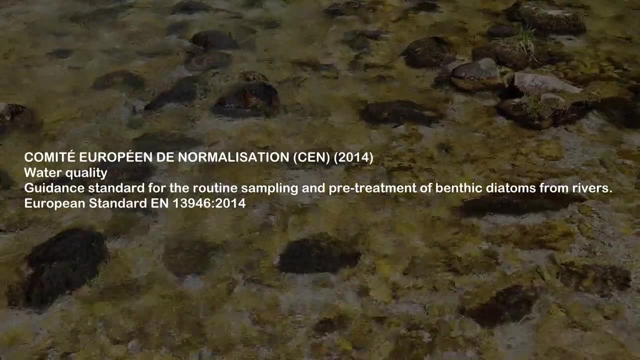 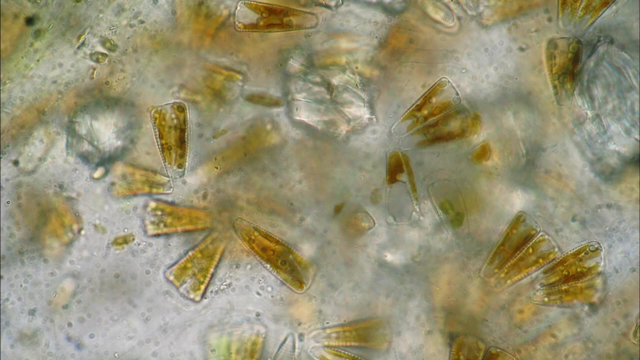 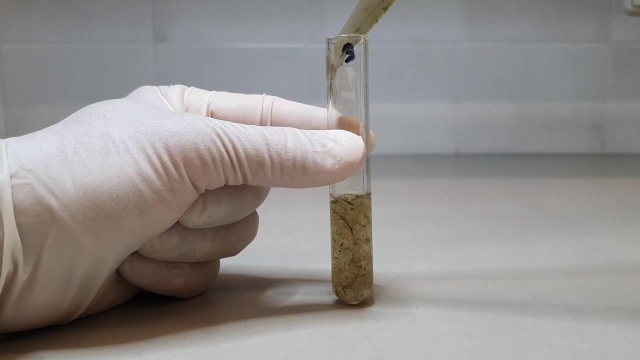 permanent slides for identification of diatoms in a light microscope. The presented procedure follows the instructions of the European standard for water quality from 2014.. For accurate identification of diatoms, it is necessary to remove all organic content from the cells. Therefore, prior to mounting, diatom samples must be cleaned by using a strong oxidizing. 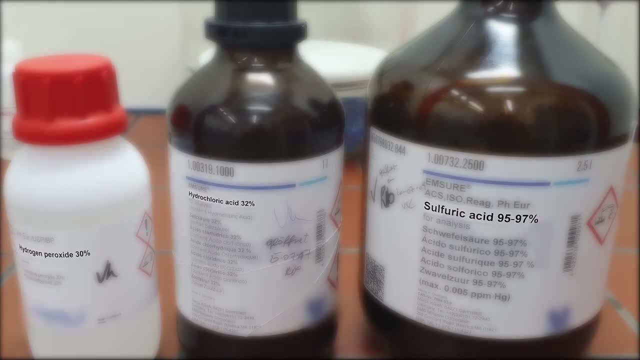 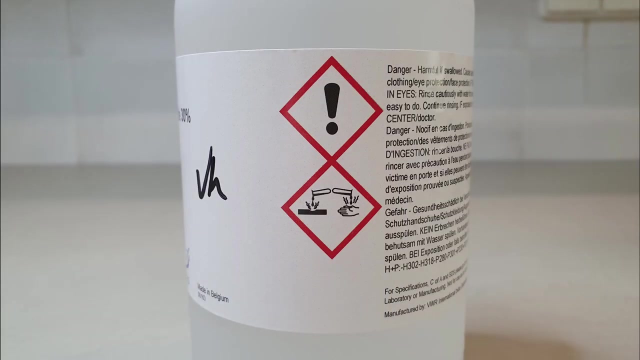 agent. The European standard mentions several methods of sampling benthic diatoms, Several oxidizing agents that can be used for the removal of organic content. In this video we are going to demonstrate the hot hydrogen peroxide method, which involves less health and safety risks and is also gentler to the diatom thrust tools. 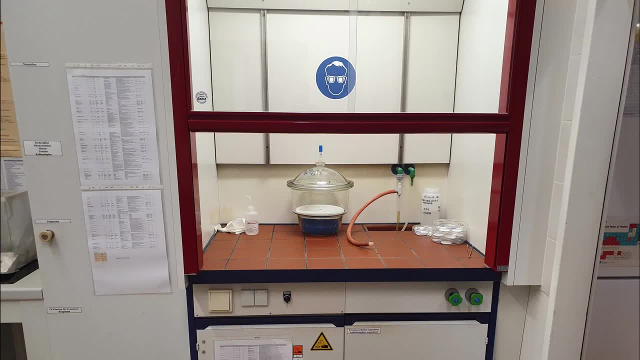 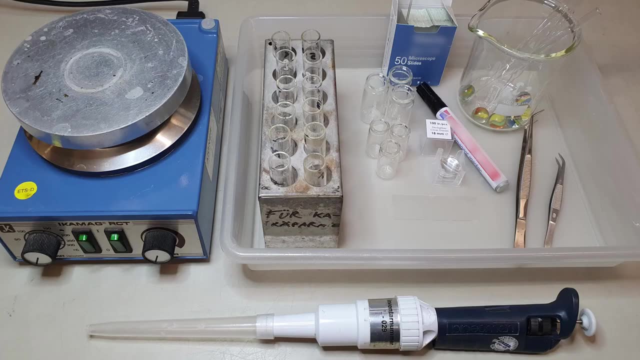 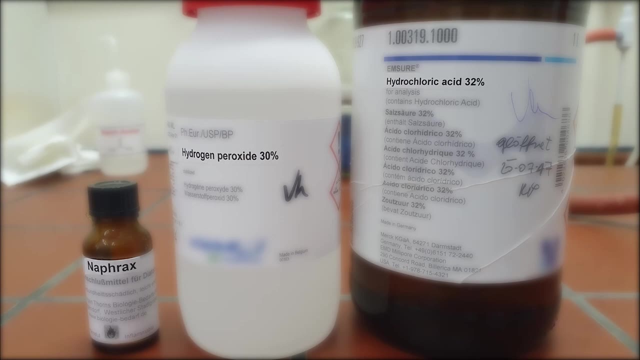 Here is the most important equipment and material we are going to use: A fume hood, a centrifuge, a hot plate, a piston operated pipette and laboratory glasswork shown in this picture. The required chemicals are 30% hydrogen peroxide, concentrated hydrochloric acid and Nafrax, as 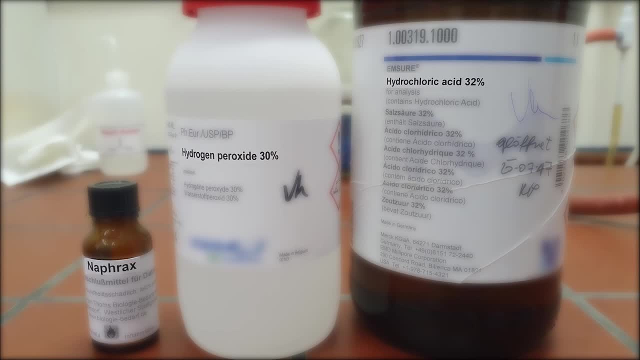 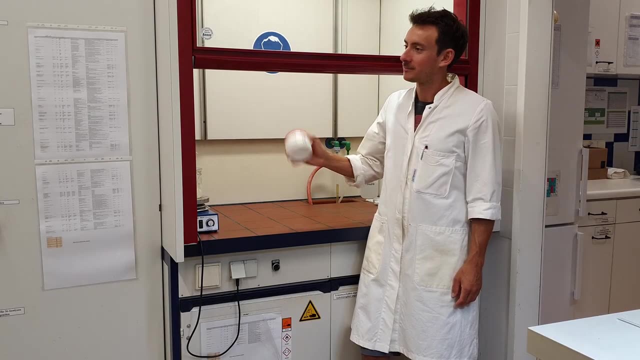 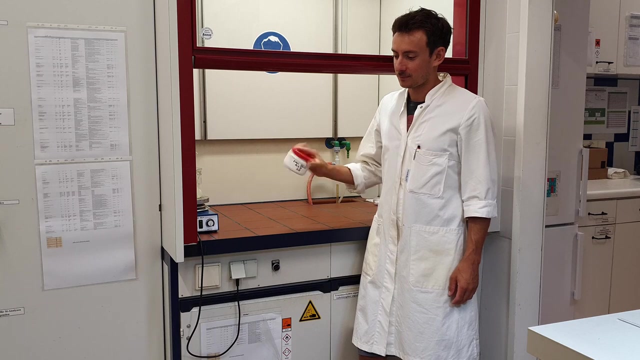 mounting media. In general, the method selection depends on the laboratory equipment and is upon operator's choice. In a first step, the collected field samples have to be well homogenized to get a representative subsample. This can be achieved by thorough shaking of the sampling container and additional mixing. 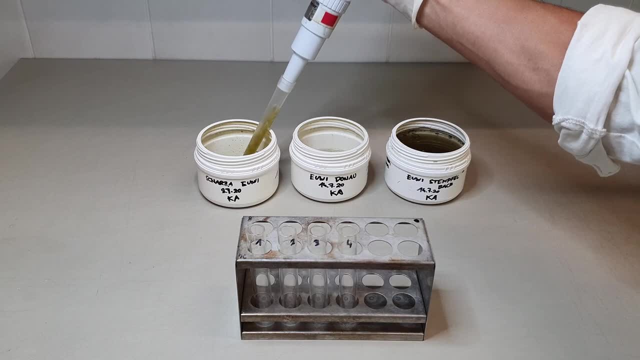 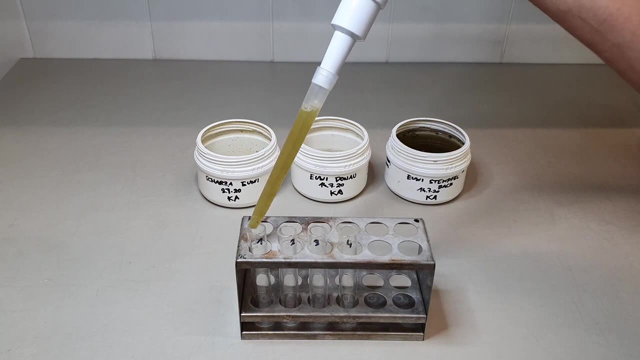 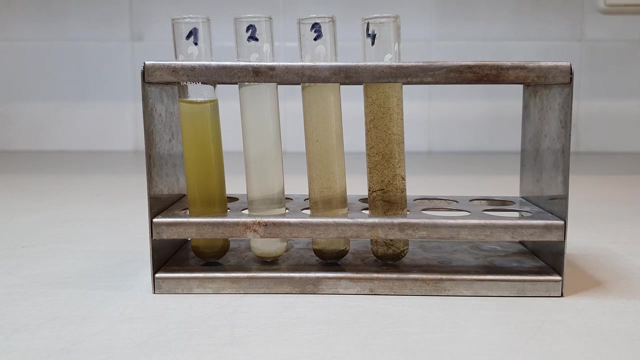 of the sample by using a piston operated pipette. Depending on the concentration of the original sample, transfer approximately 10 mL of diatom suspension into a centrifugation glass tube. If the sample is not sufficiently concentrated, the subsample can be further concentrated. 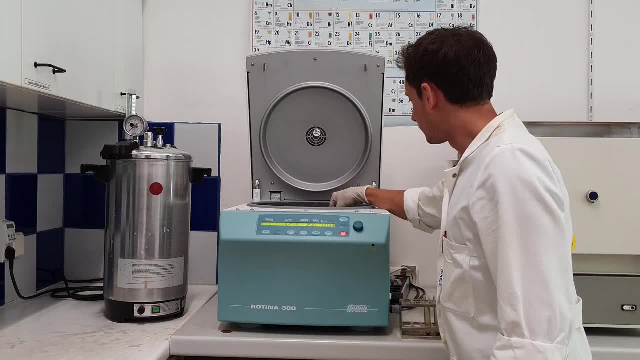 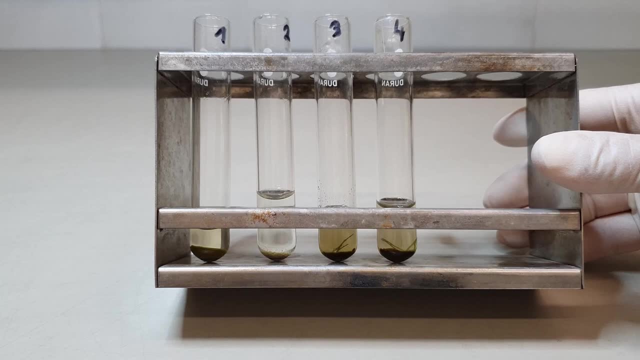 by decantation or centrifugation and addition of more sampled material. The goal is to obtain 2-3 mL of concentrated diatom suspension to start the cleaning process. The sample can be further concentrated by decantation or centrifugation and addition. 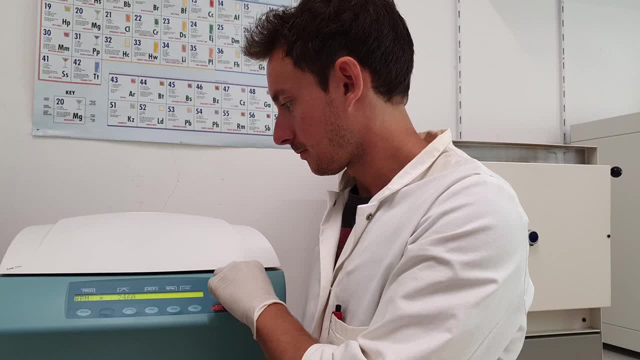 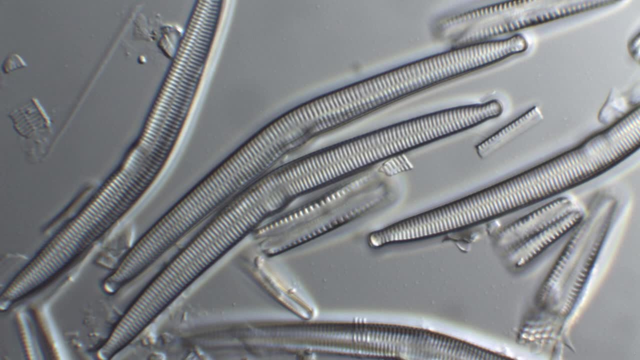 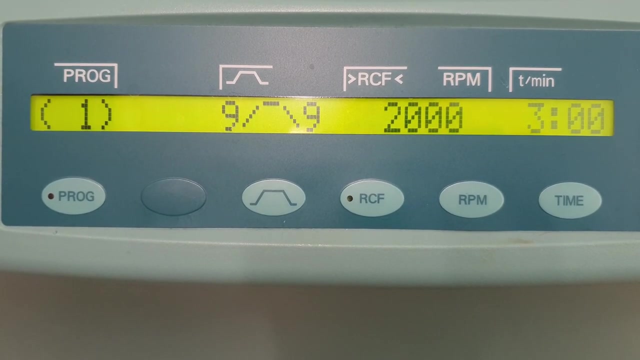 of more sampled material. When using a centrifuge, make sure that the centrifugation settings do not exceed 2500 rotations per minute. otherwise long-penned diatoms are likely to break. We recommend to centrifuge at 2000 rpm for at least 3 minutes. 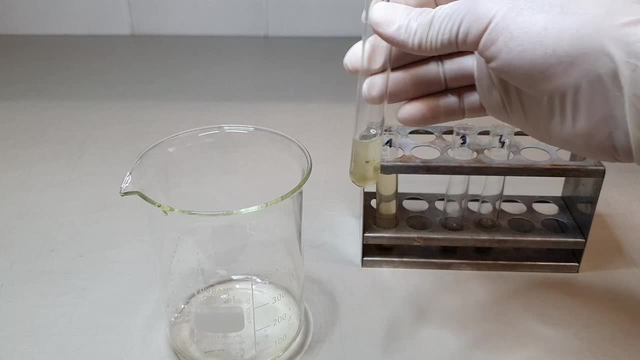 After centrifugation: decant the supernatant with a quick movement of your hand to not lose any sedimented material. Alternatively, you can also use a supernatant. You can also use a supernatant with a quick movement of your hand to not lose any sedimented. 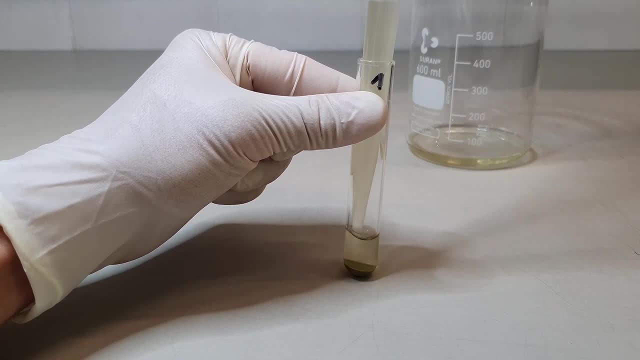 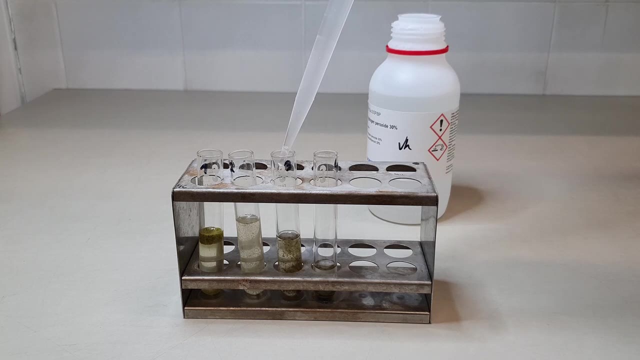 material. You can also extract the supernatant by using a pipette. In the next step, we use hydrogen peroxide as a strong oxidizing agent to remove all organic content from the diatom cells. For this purpose, pipette at least 3 mL of hydrogen peroxide into each glass tube. 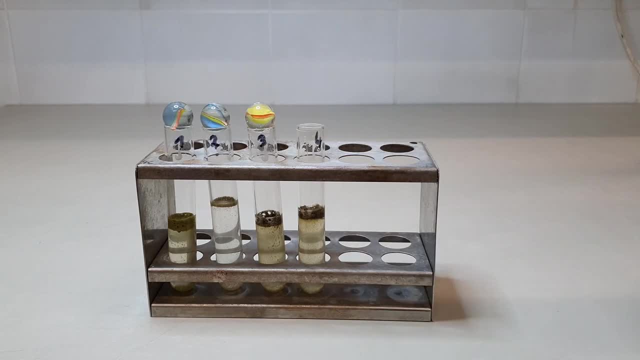 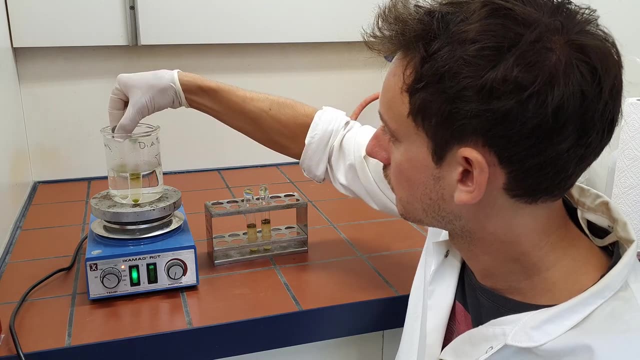 Since the reaction starts immediately, the glass tubes are covered with glass beads to avoid spilling of material. Transfer to the next step. We can also extract the supernatant by using a pipette. Transfer the glass tubes to a beaker with hot water and heat for approximately 2 hours. 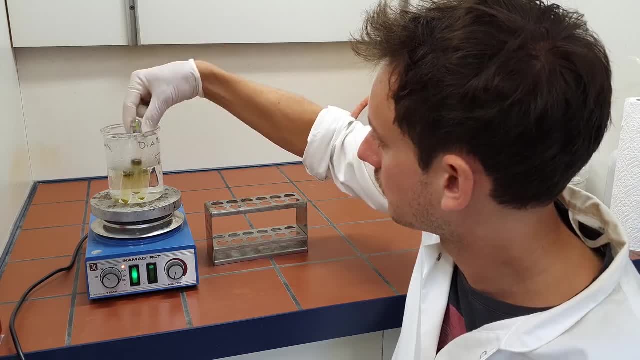 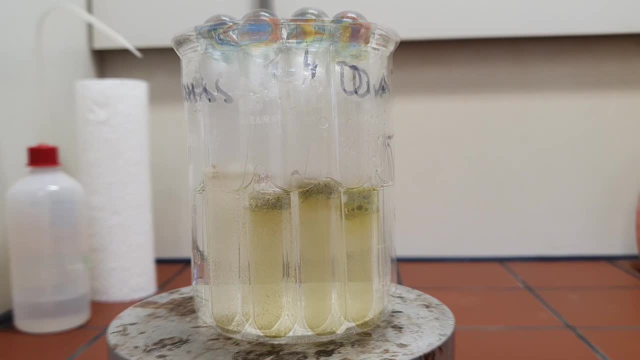 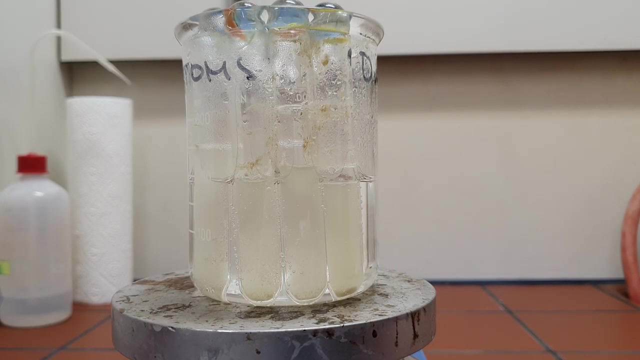 at 100°C. Depending on the organic content of the sample, it takes around 1-2 hours until all organic material is oxidized. As a result, the reaction dies down and the material is bleached out. If some organic content remains, even after 2 hours of boiling, add more hydrogen peroxide. 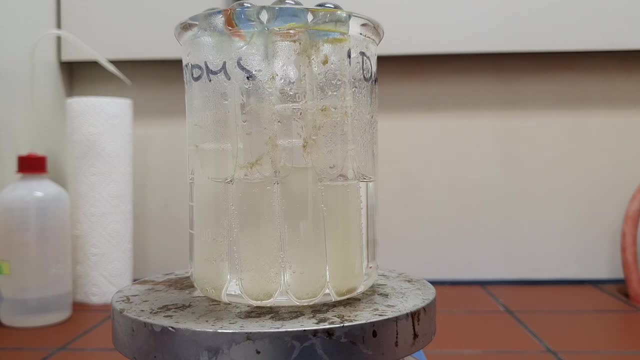 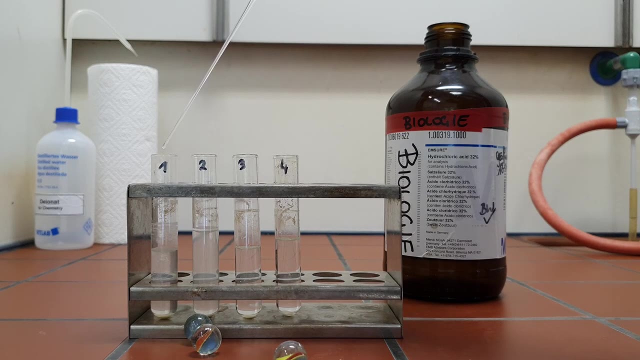 and continue with the reaction until all organic material is removed. We can also extract the supernatant by using a pipette. When there is no more visible reaction in the tubes, remove the tubes from the bath and add 3-4 drops of concentrated hydrochloric acid to the samples. 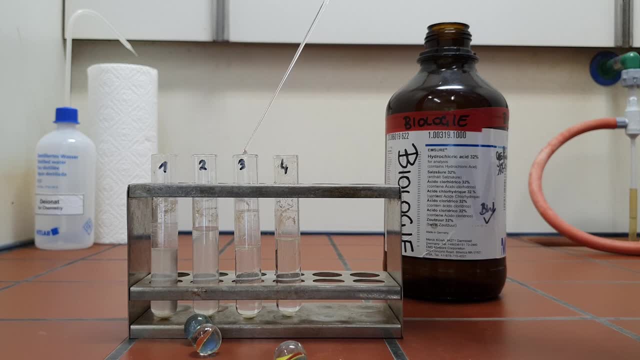 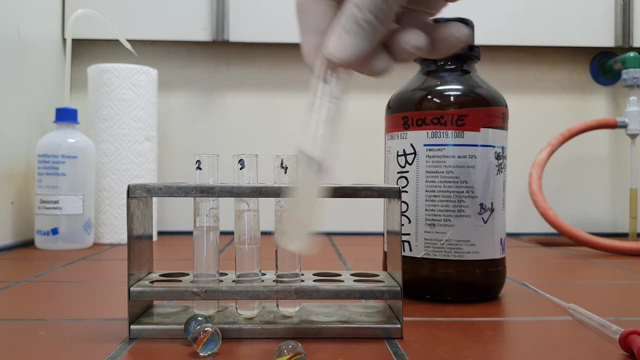 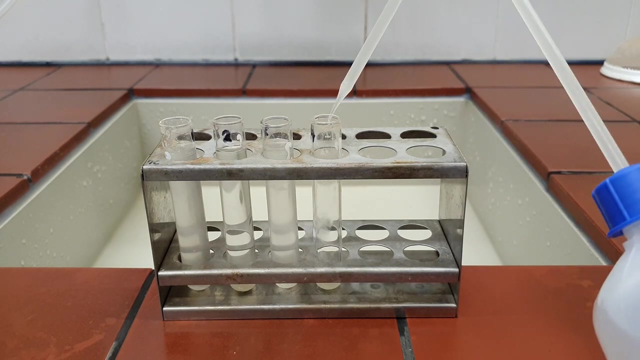 This eliminates the remaining hydrogen peroxide and any carbonates or calcareous precipitates. Mix the samples and let them cool down for at least 30 minutes until the reaction stops. In the last step, rinse the diatom suspension 3 times with distilled water to remove any 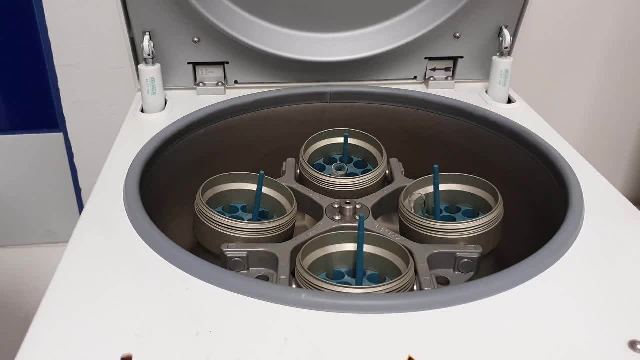 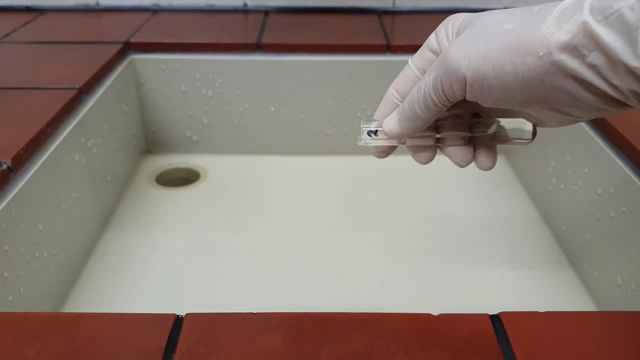 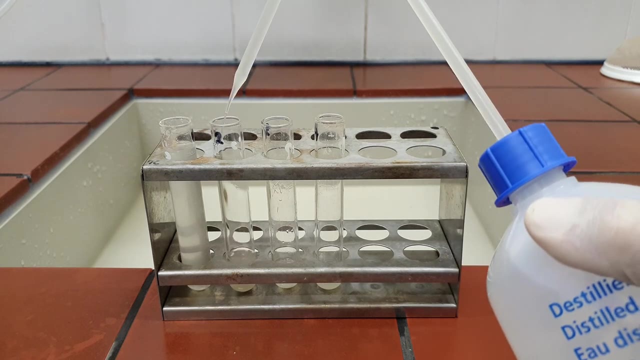 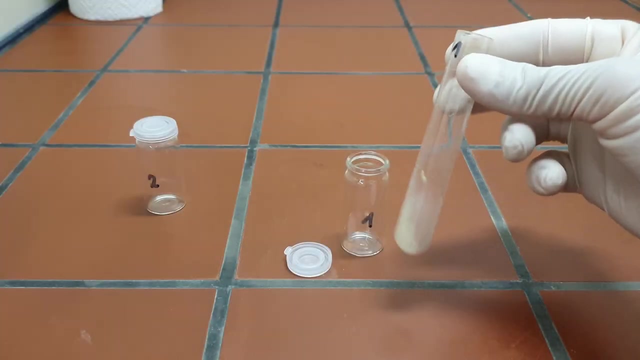 chemicals from the sample. In order to do this, centrifuge the samples at 2000 RPM for 3 minutes, decant the supernatant, add distilled water and repeat the procedure again. Finally, transfer the cleaned and rinsed diatom suspension with a small amount of distilled 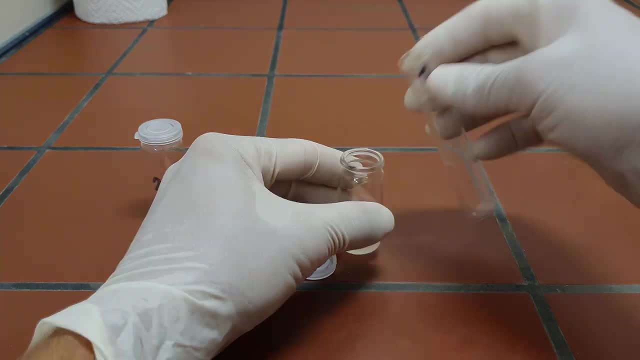 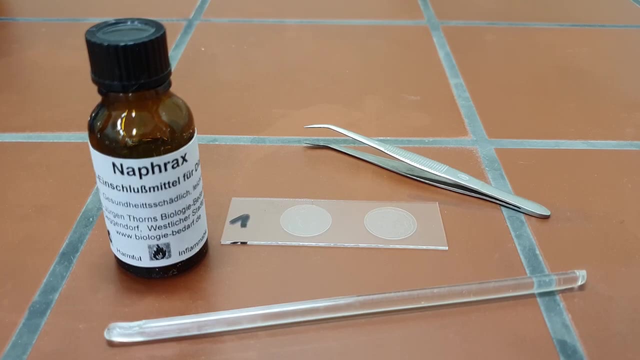 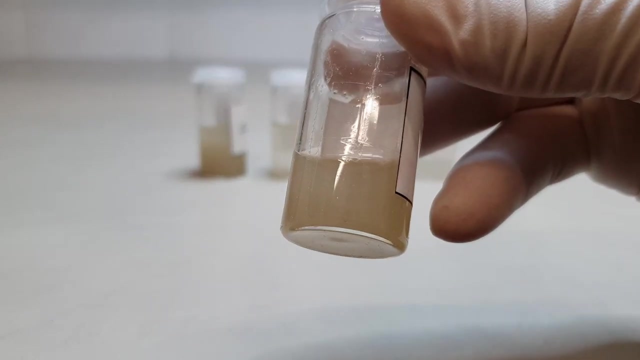 water into a lathed container. This is the final result For identification in the light microscope. the diatom valves still need to be mounted onto a permanent slide using a mountant with high refractive index. The cleaned diatom suspension is too concentrated for mounting and therefore needs to be diluted. 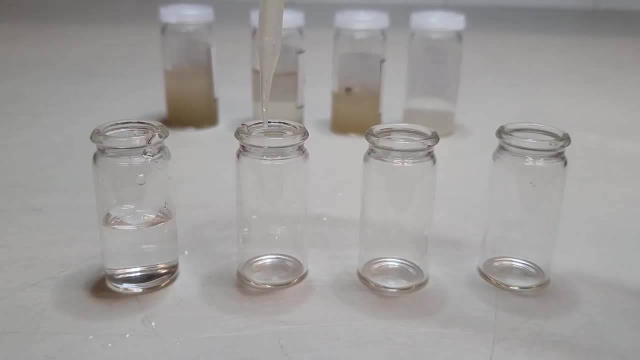 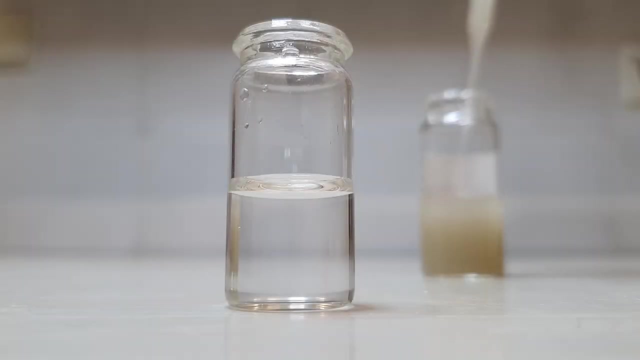 first, Prepare a glass vial filled up halfway with distilled water. Homogenize the diatom suspension with a pipette and transfer a few drops of the suspension to the glass vial. The diluted suspension should be only slightly milky, with fine particles being just visible. 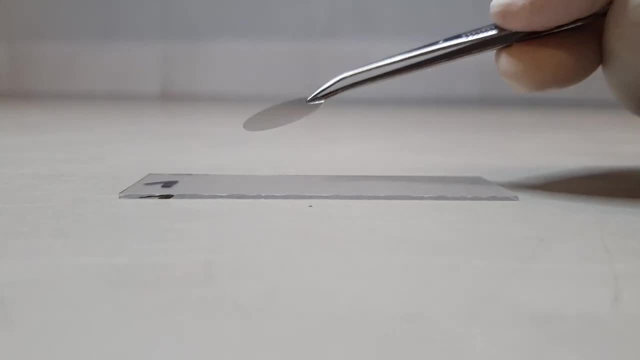 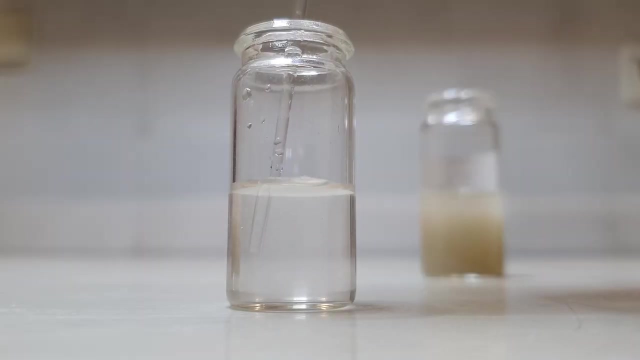 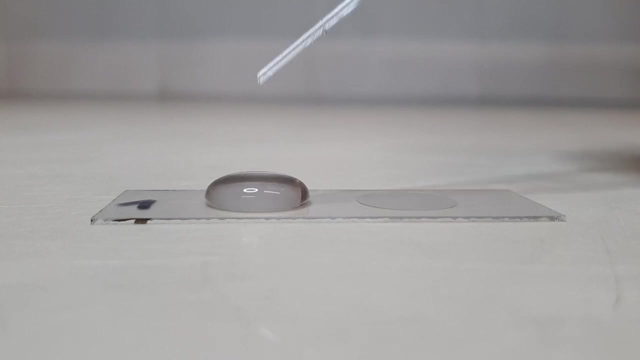 when held up to the light. Place two coverslips onto a microscopic slide, Homogenize the diluted suspension and carefully fill up the first coverslip with the diluted sample To obtain a second subsample with 3 times larger suspensions. just slide it into the. 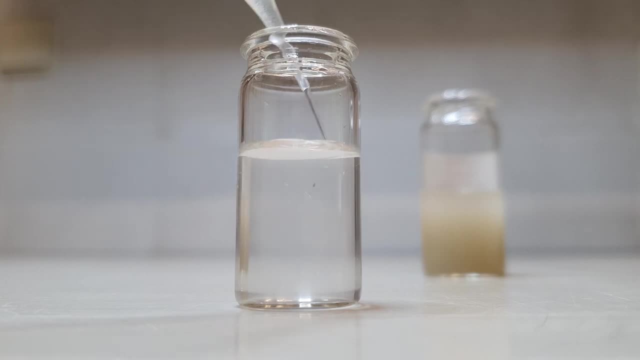 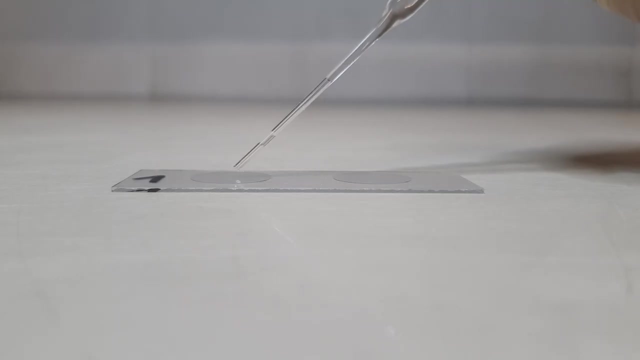 with different concentration. fill the glass vial all the way up with distilled water and repeat the procedure with the second coverslip. Alternatively, you can also transfer different volumes of the diatom suspension onto the coverslips. We recommend letting the coverslips dry overnight at room temperature to evenly 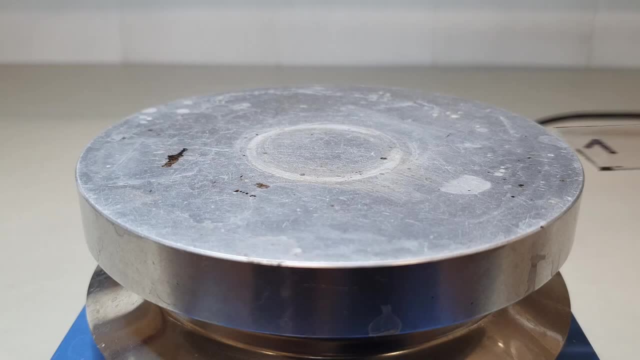 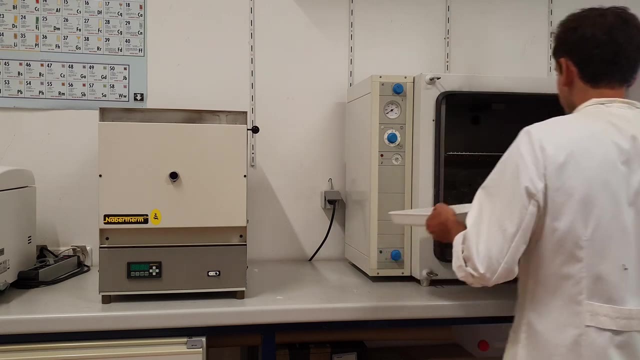 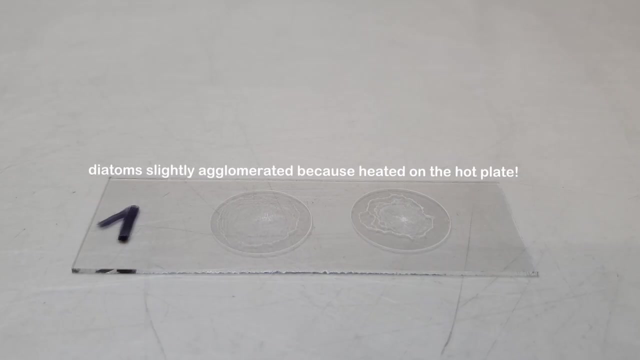 spread the diatoms over the coverslip. When time is limited, a hot plate or a drying oven can also be used to speed up the process, but consider that diatoms tend to agglomerate when drying at elevated temperatures. Once the coverslips are dry, they are ready for mounting. 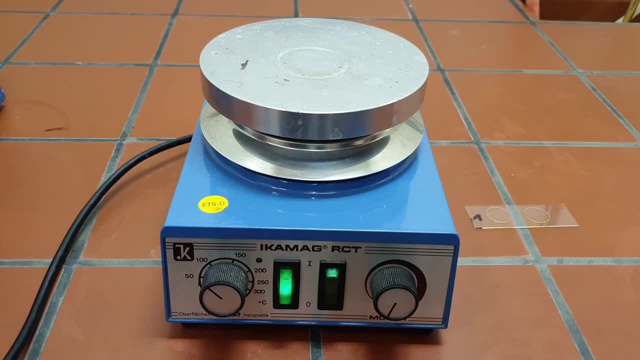 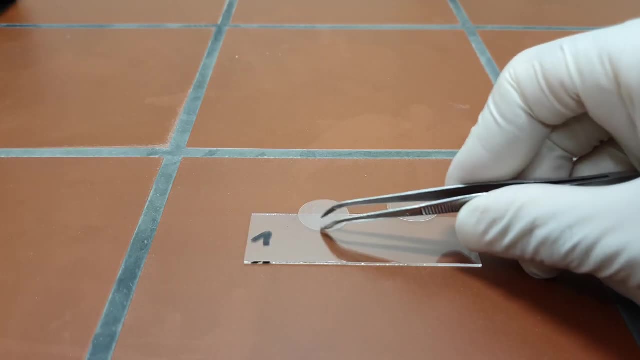 This must be done in the fume hood. Preheat a hot plate in the fume hood to 110 degrees celsius. Place one to two drops of Nafrax onto the coverslip. Place the hot plate onto the microscopic slide using a glass rod and invert the coverslips with. 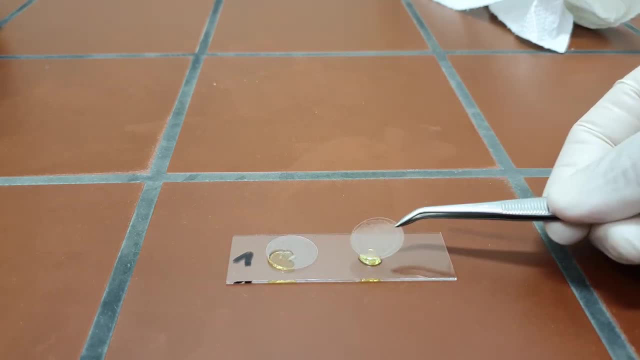 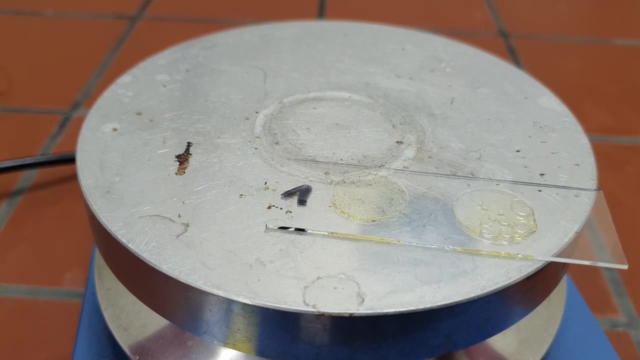 the dried diatoms quickly onto the drops of Nafrax. The microscopic slide is then placed on the hot plate for around two minutes until the solvent is evaporated. When no more bubbles are forming, move the slide from the hot plate onto the workbench and quickly but gently press down.